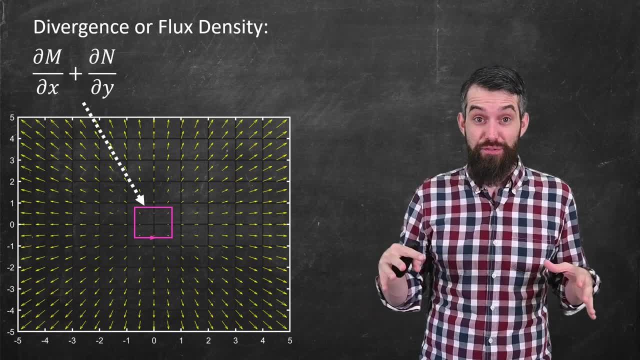 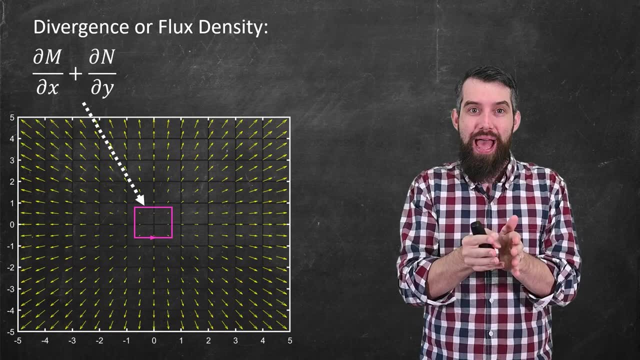 to y. If I think of my field, for example, as being a velocity field- and I've got some region- I'm going to be asking the tendency for the field to pour out across this tiny, tiny little path. It didn't even matter where the path was. I happened to previously put it at the sort of origin, but 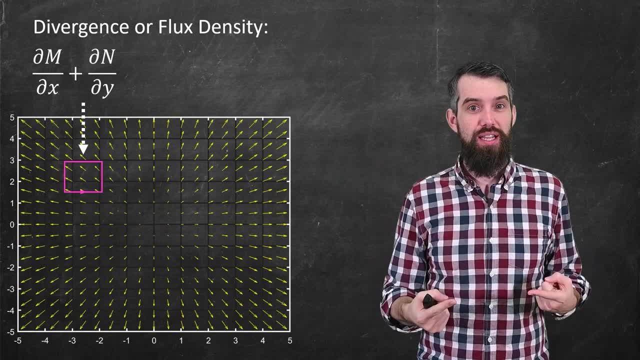 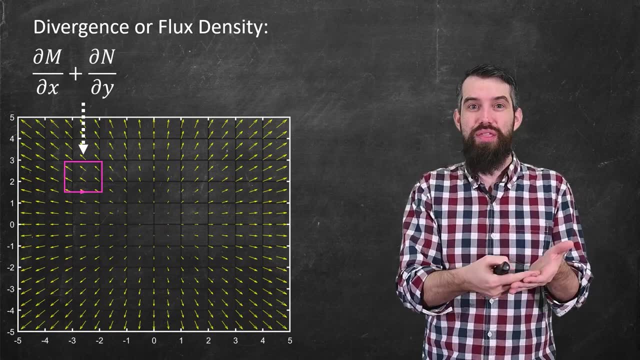 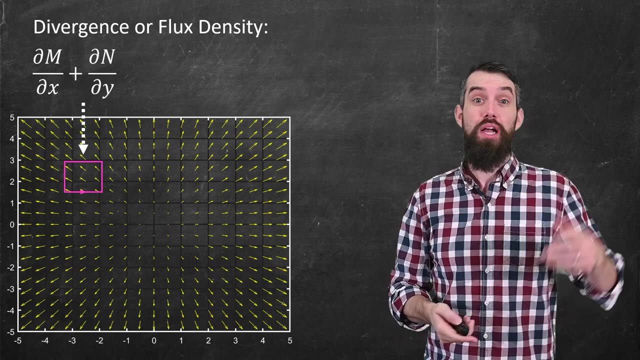 at any spot you could compute the divergence. For example, even at this off-center point there is a positive divergence because the arrows that are pointing into this little path are shorter than the arrows that are leaving from it, and so a net outflow or positive divergence, Okay, so going back, 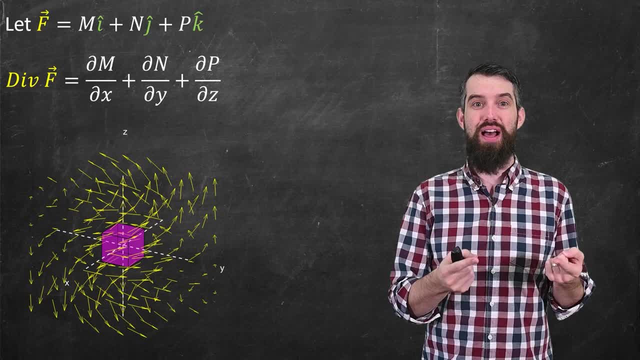 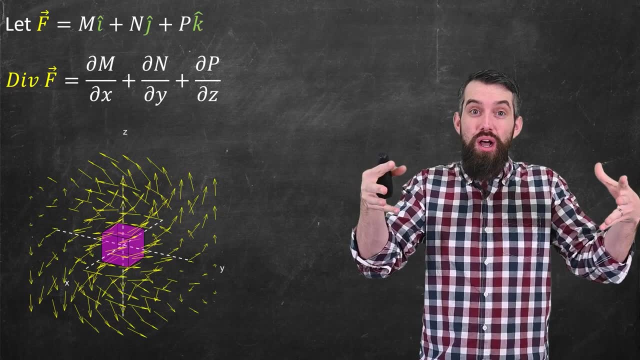 to the three-dimensional case. the idea here now is, instead of a little square, I have a little cube and I'm asking: to what degree is the vector field spreading out across the boundary of this little cube? And as you investigate different points and thus are investigating, 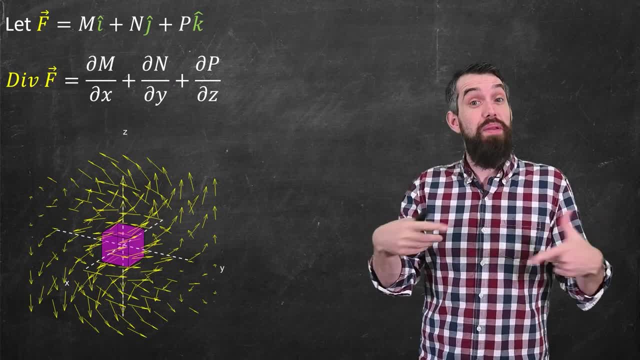 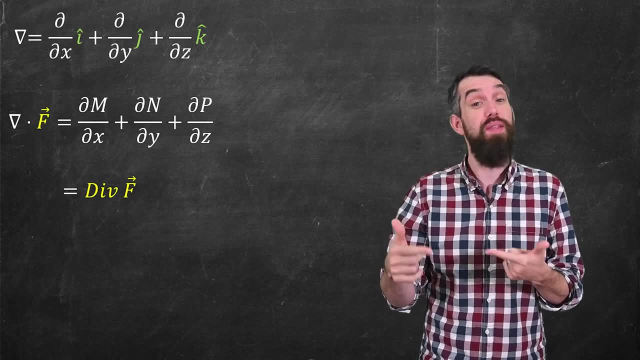 different little tiny boxes. the divergence may be different at different points along the field. Now we can actually simplify the expression for divergence in much the same way as we simplify the expression for curl. We have a del operator which is just the partial respect to x in the i. 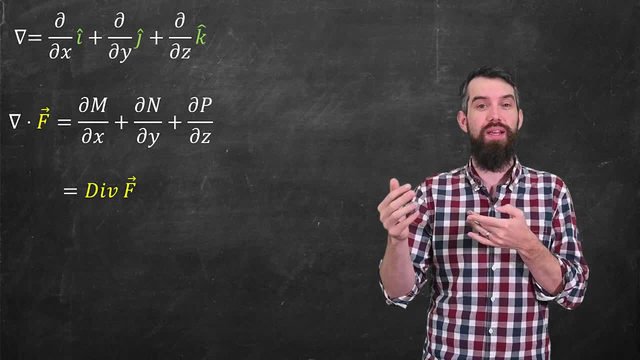 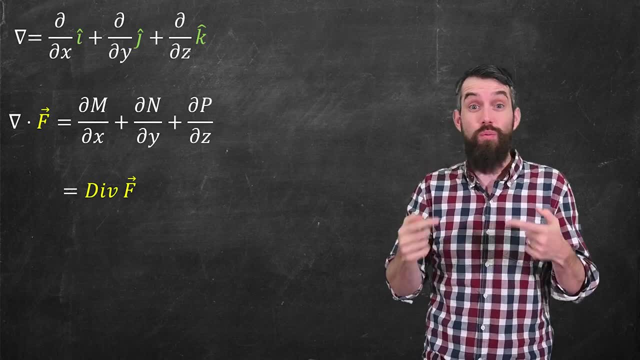 hat, the partial respect to y in the j hat and the partial with respect to z in the k hat. Then, if I take the dot product of this del operator with the function of the dot product, of the dot product of the field f, then what do I get? Well, precisely, the divergence: the partial of m with respect to x, the. 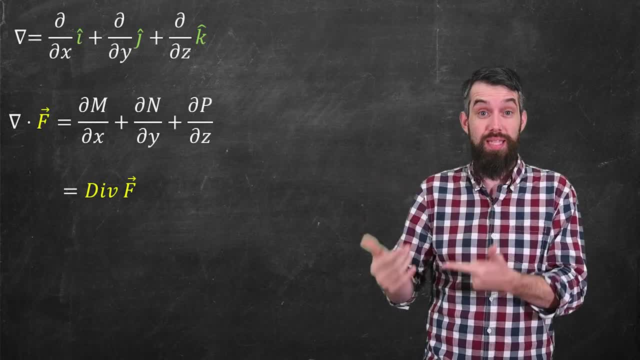 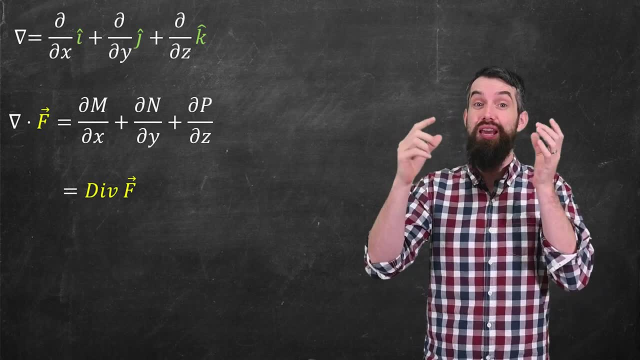 partial of n with respect to y and the partial of p with respect to z. This is an operator, which means: is it something that takes a function, transforms it to another function? in this case, it takes a vector function, capital f- and spits out the vector function, the divergence of f. 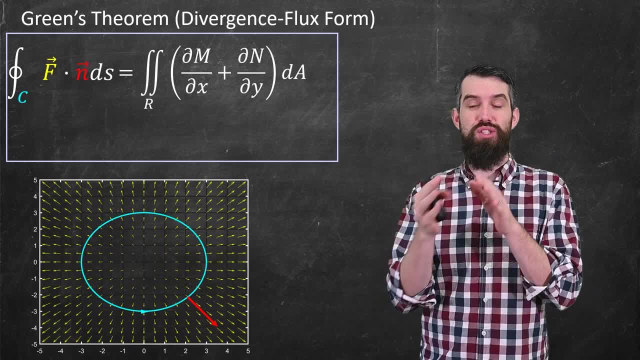 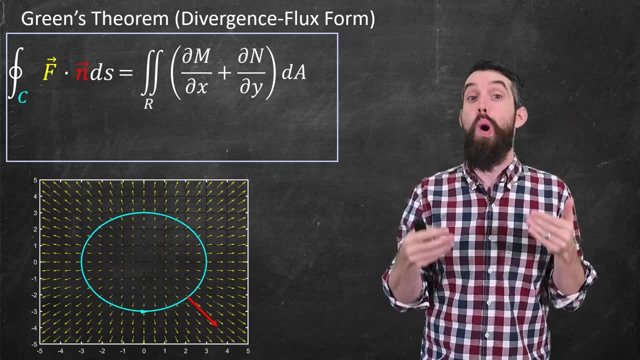 Now let's go back and review Green's theorem in its divergence or flux form. When we previously talked about Stokes' theorem, we saw that Stokes' theorem was a generalization of one half of Green's theorem. Today, in this video, the divergence theorem is going to be the generalization of the other half. 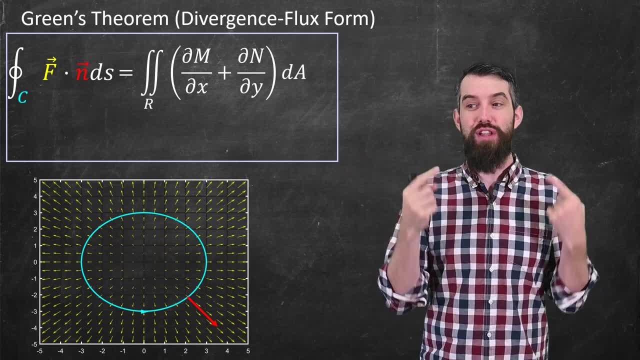 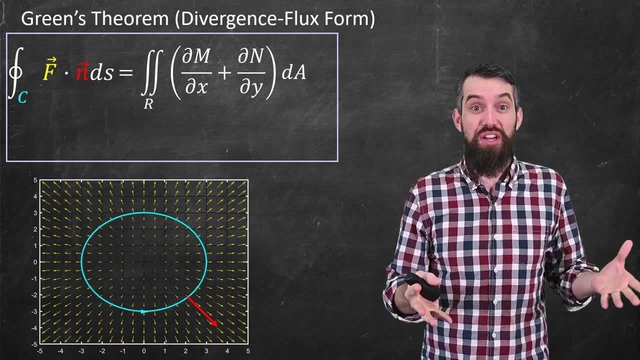 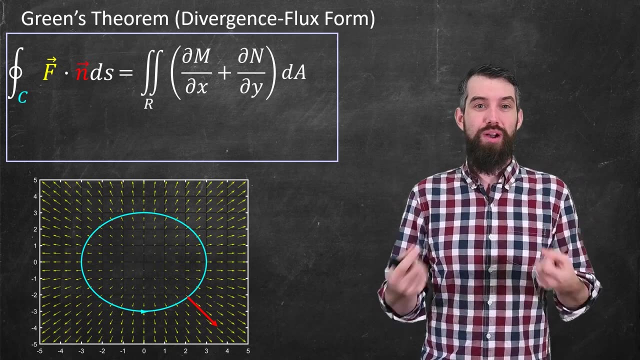 of Green's theorem. So Green's theorem in its divergence or flux form is all about the flux across a curve. So I'm imagining now I have a bona fide curve, not the small little infinitesimal one we used to have an actual big curve. It's got a normal vector at any point and the question is: 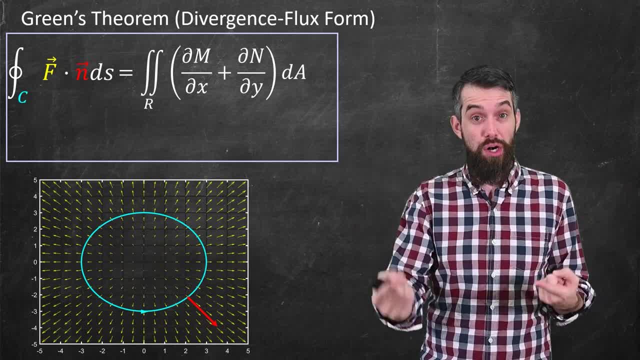 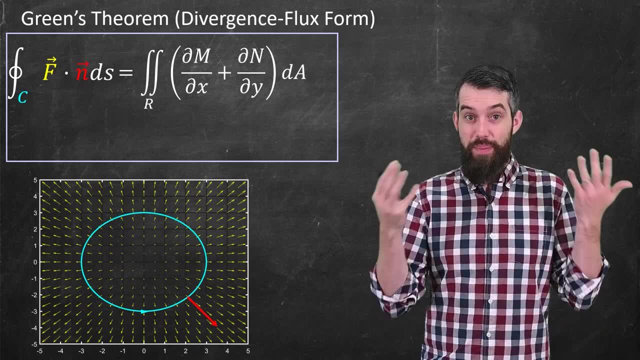 well, how much is the field spreading out across the curve? Well, the question is well, how much is the field spreading out across the curve? Well, the question is well, how much is the field spreading out across the boundary of this curve? How much is the field aligned normal to this curve? And so what we have is this comparison. 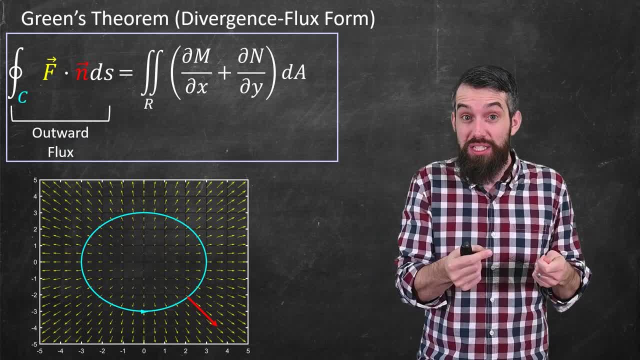 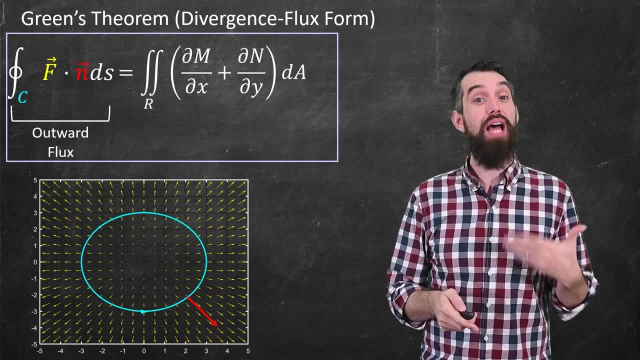 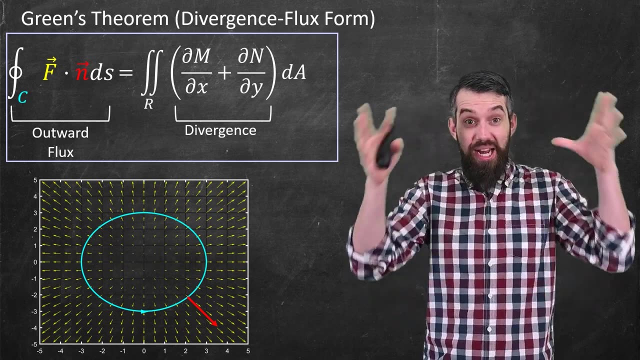 between the boundary. in other words, I'm asking the outward flux across this boundary curve. and then what Green's theorem does is: it relates this to a double integral over the entire region of the divergence or of the flux density? The basic argument is, if I imagine cutting up the 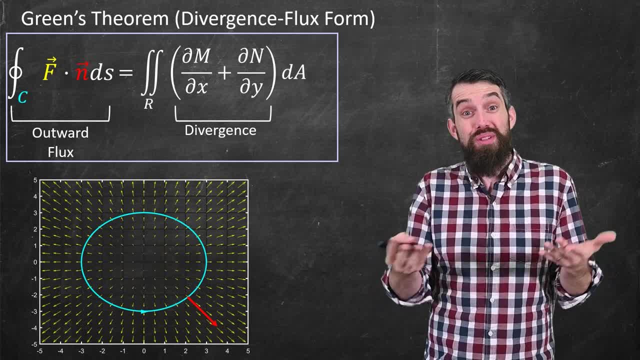 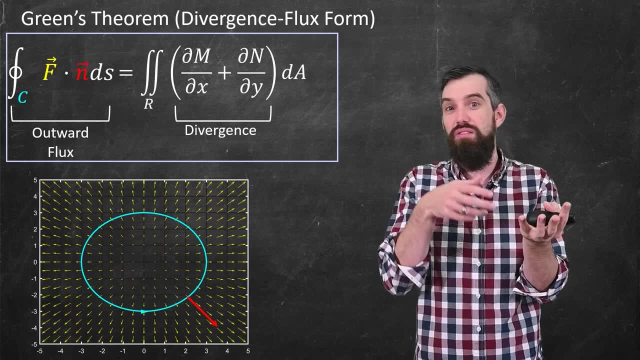 big region to a whole bunch of small little pieces. in the interior there's a ton of cancellation And the idea is, if you have two adjacent regions, the flux from the left to the right is just the negative of the flux from the right to the left, And so adding. 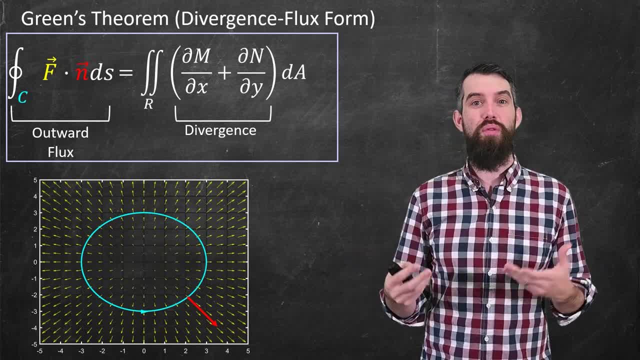 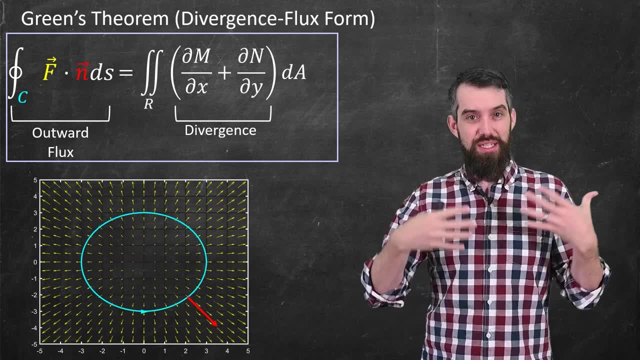 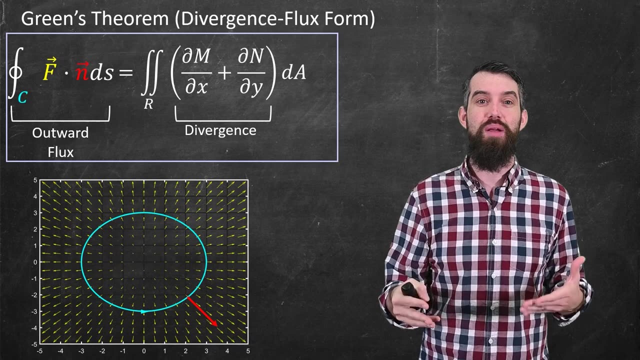 everything up would just make that cancel. So when you get rid of all the interior cancellation of this divergence, what's left is that crossing out the final boundary which gives us the outward flux. Now we get to do something new because we have an improved terminology for talking about. 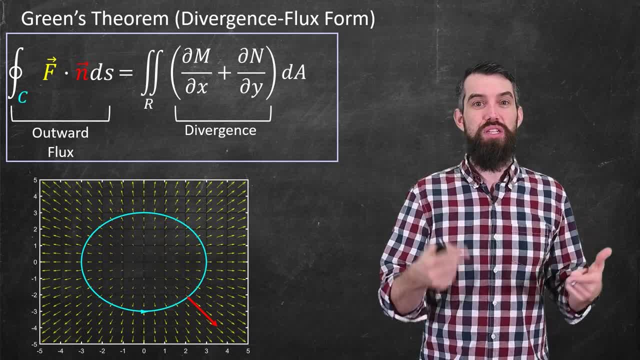 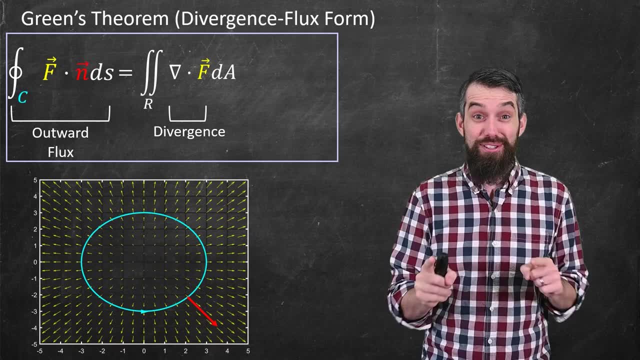 the divergence. We saw that. the gradient of f: we saw that del dot f represented the divergence. So I'm just going to replace that in my formula here. Okay, now it's time finally to upgrade from the two-dimensional situation where Green's 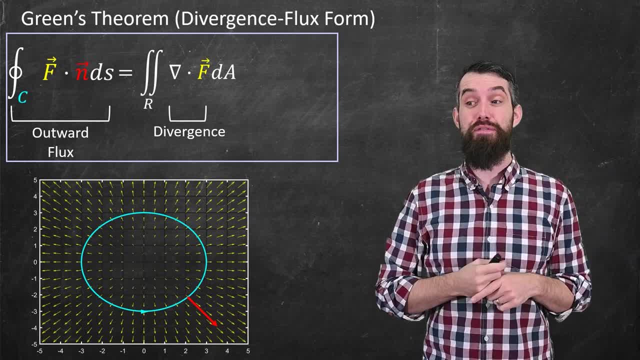 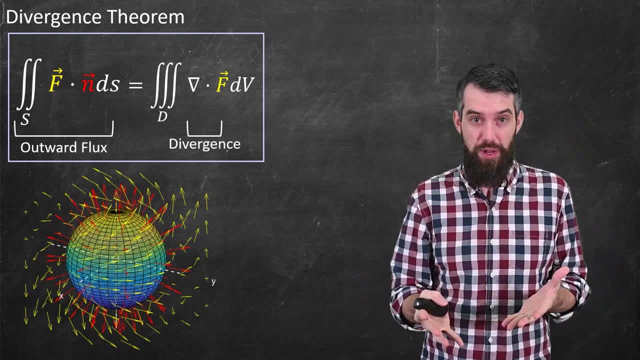 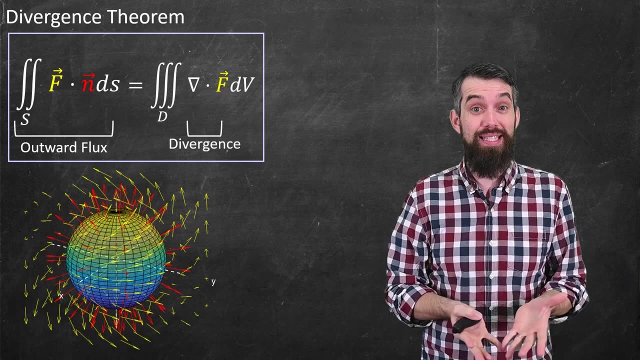 theorem applies to the three-dimensional situation of the divergence theorem. So what's going on? Let's look at the picture first. In the picture I have, in yellow, just a vector field. Living within that vector field is a surface, and I've plotted the surface of a sphere as my example of a. 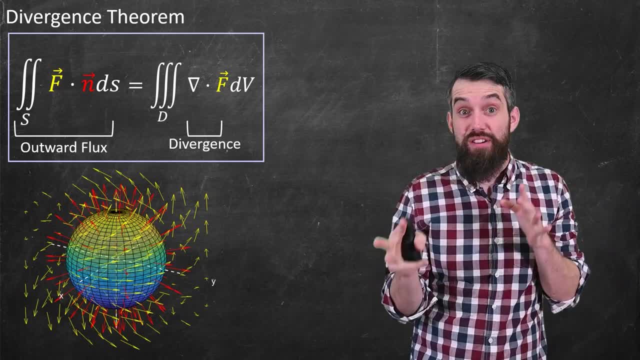 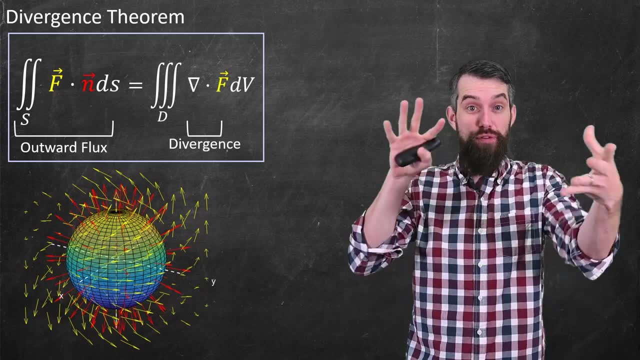 closed surface. And then I've also plotted a lot of red vectors. What are those? The red vectors are normal to the surface. You have your surface. This has a whole bunch of normals at every point, And then that whole thing lives within the yellow vector field. Okay, so what happens to the actual 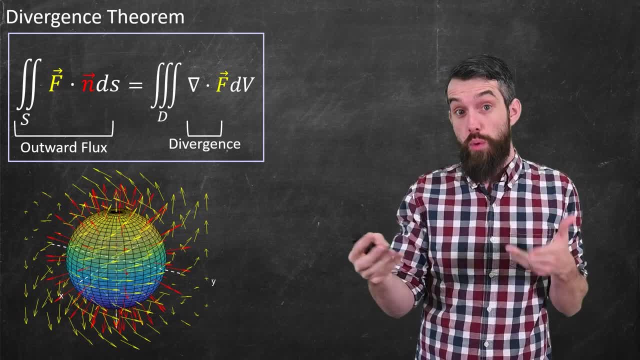 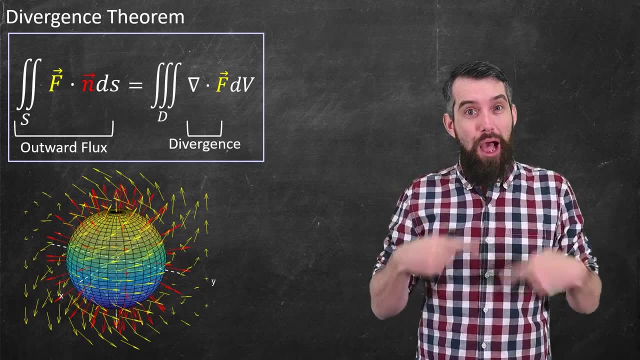 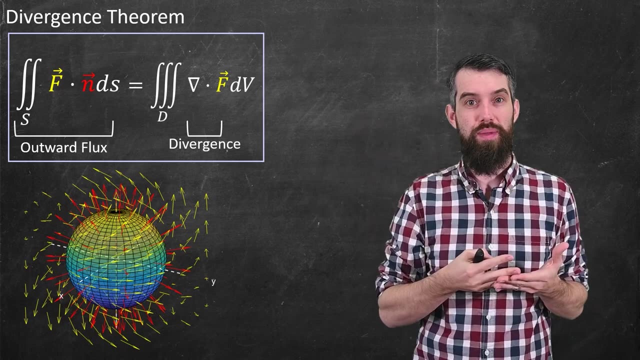 formula. Well, the left-hand side still represents the outward flux, but it's a completely different formula than it was before. Previously it was the outward flux across a curve, but now I'm talking about a surface. So the left-hand side of the divergence theorem is a surface interval. And then 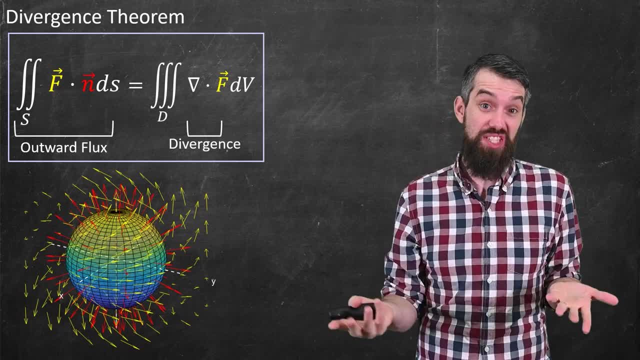 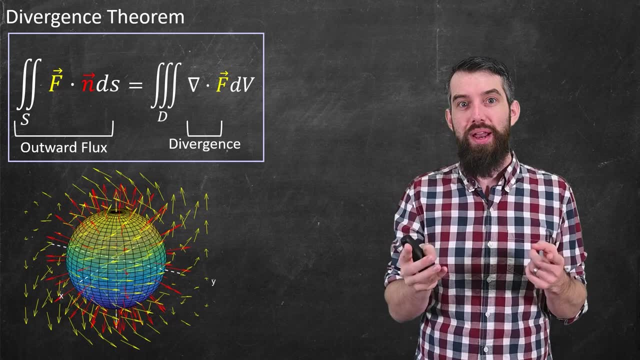 the right-hand side also changes. The integrand is actually the same thing. it's just the divergence. Now the divergence would be the sum of three things versus the sum of two things, but still just the divergence. But now the interior of a surface is a volume, and so it is a triple. 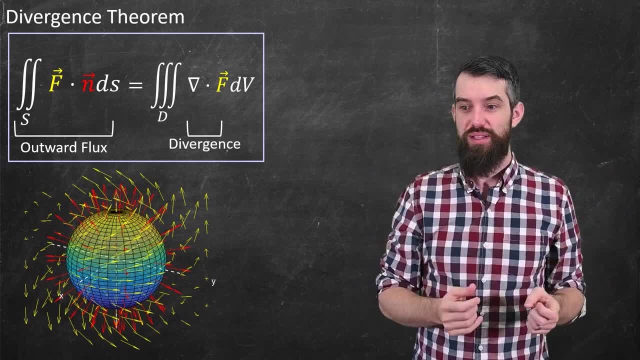 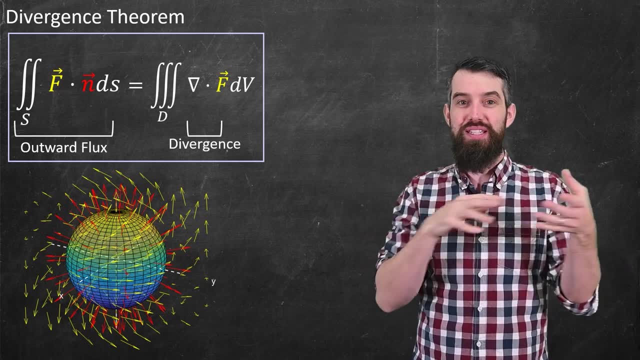 interval with respect to a volume of the divergence. So I'm imagining that I have a domain. The boundary of the domain is going to be a surface. I'm going to take the interior of the surface and I'm going to add up, all through the interior, all through that volume, the tendency for the vector field to 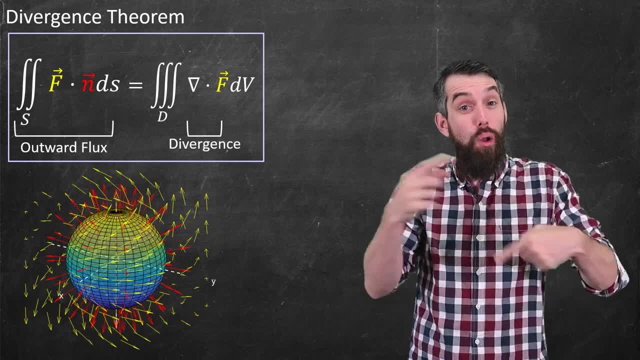 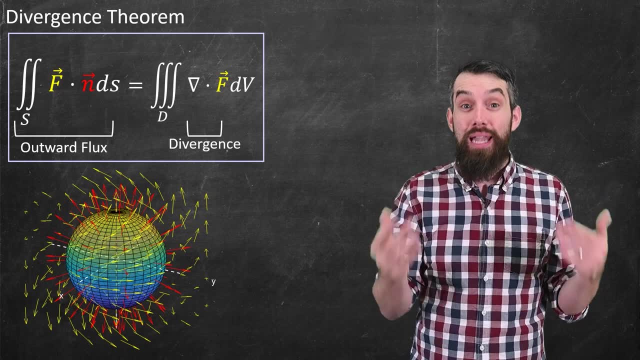 disperse at a point, for there to be divergence at a particular point, All in the middle we get interior cancellation. So then, when all of those divergences are added up, everything in the middle cancelling, what we're left with is just the portion that can't cancel the portion. 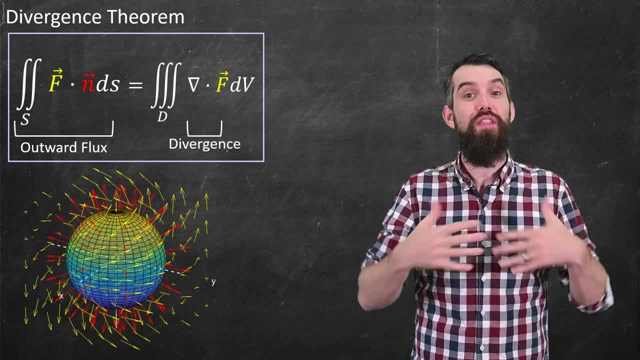 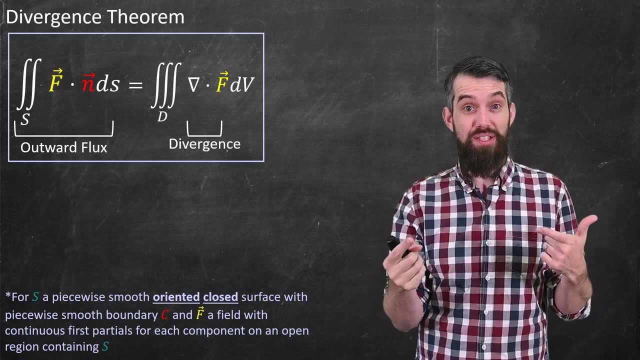 along the boundary, which in this case is a surface, And we get the outward flux across that surface. Now I need to be clear about what the condensate is. So the condensate is the surface. So we're talking about a surface and the surface needs to be nice in the sense of being. 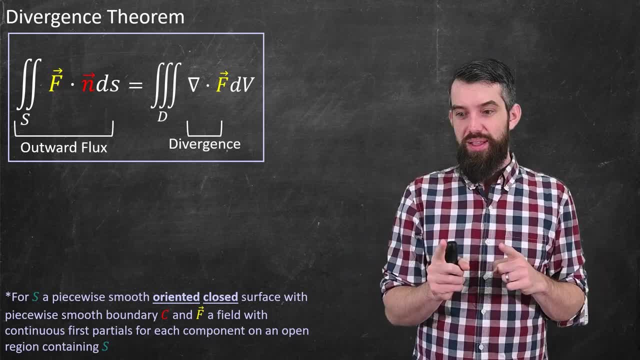 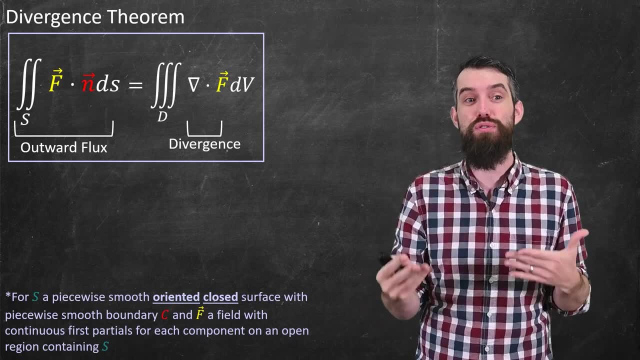 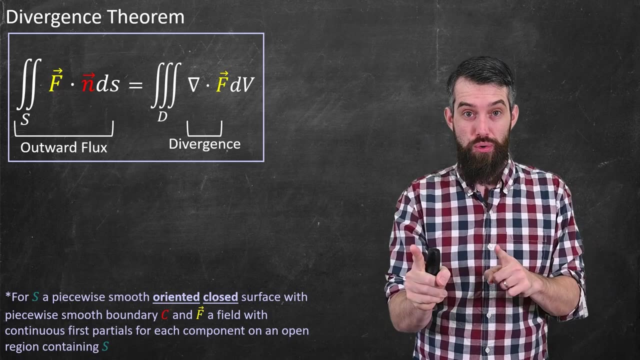 piecewise, smooth, like a sphere or a cube. But in addition it needs to be both oriented, which means it has two different sides, a continuous specification of those normals so that I can actually make sense of outward flux, make sense of f, dot, n. But in addition it needs to be closed. 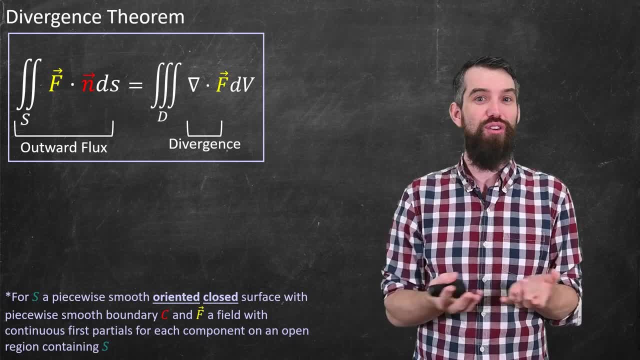 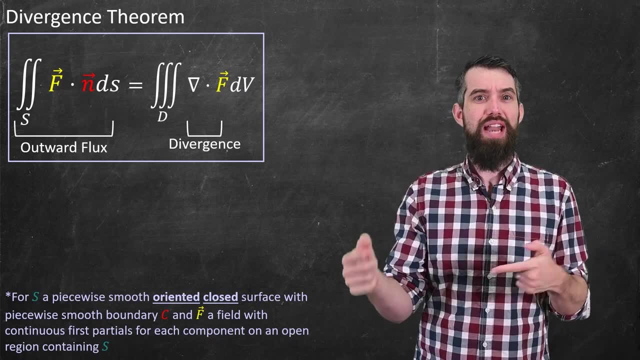 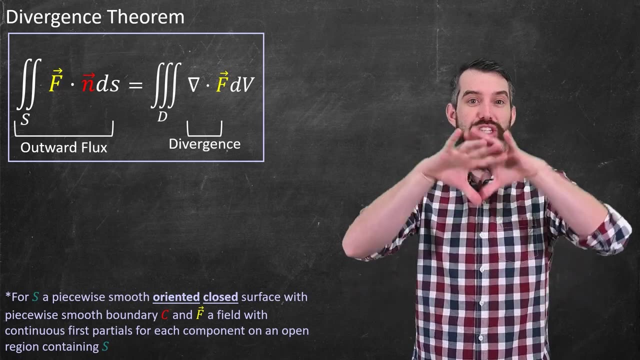 That is the divergence- doesn't make sense for, for example, a bowl with an open top. It has to be something that completely closes a region. This is somewhat analogous to in Green's theorem. We also demanded that our curves were closed here and thus contained an area. Now we're imagining 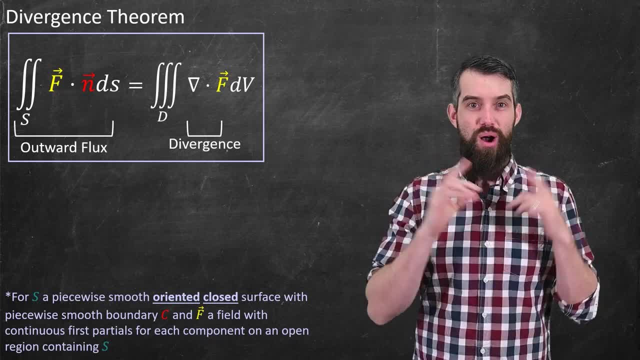 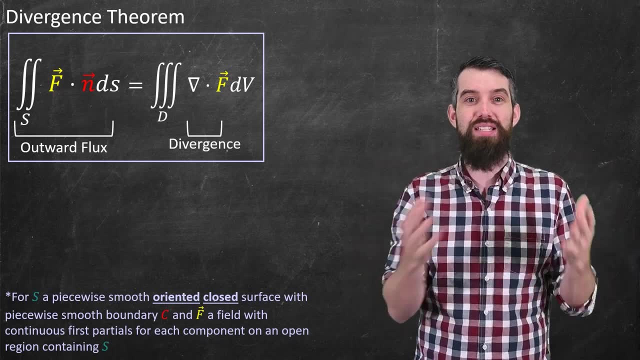 our surface is closed and thus containing a volume. All right, so that was the divergence theorem Coming up. I need to do some examples, for sure, but I also want to do a video that unifies the divergence theorem, Stokes' theorem, Green's theorem and the fundamental theorem of calculus.